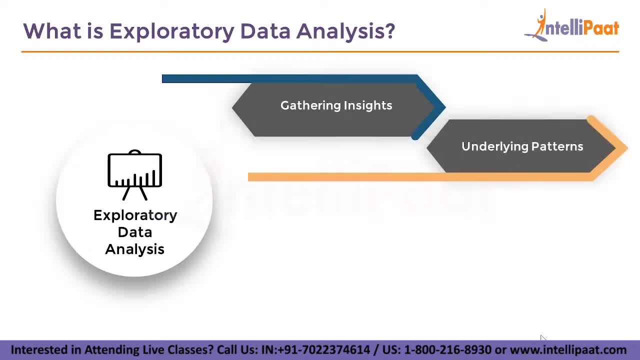 These insights may include the pointers that best explain the distribution of the data points, peakness and other necessary information like relationship between each of the variables in the data. You are able to identify the underlying patterns which you may not be able to identify just. 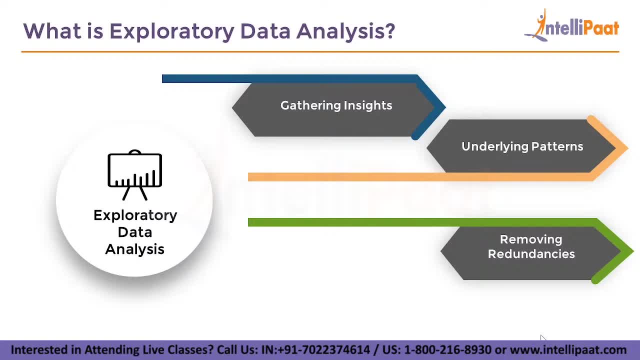 by looking at it, You are able to remove the redundancies, like null values and outliers. The idea is to use the processes and tools available to us to make sure that no stone is unturned when it comes to exploring the data. The main objective of the EDA is to understand which kind of solution or if we are using. 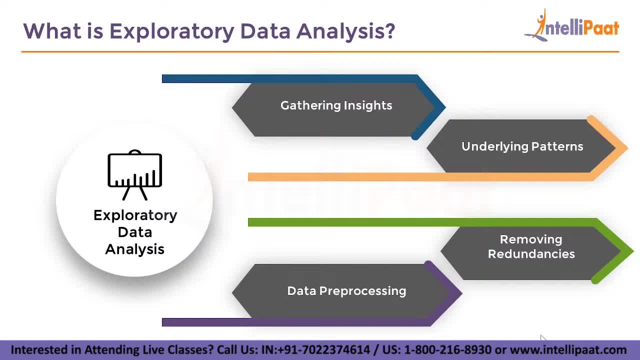 the machine learning approach we are going to use to solve the problem. This practice gives us enough room to decide the outcomes Based on the findings while doing the EDA. Now that we have a vague idea about what exactly is exploratory data analysis, let's go ahead. 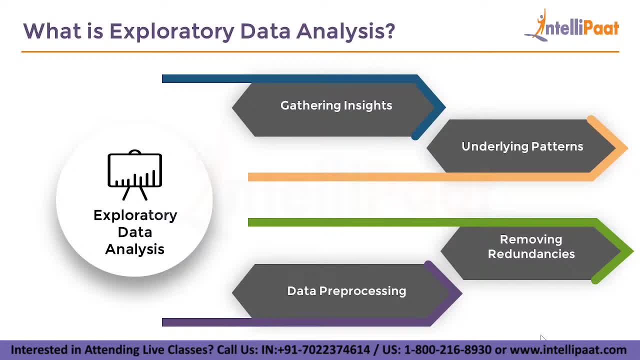 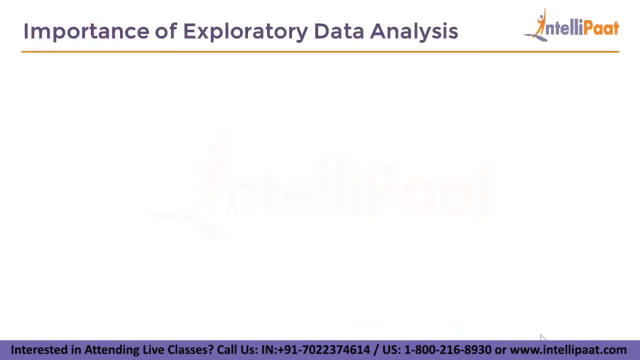 and look at why it is so important for any aspiring data scientist to be thorough with the concept of EDA. So when we discuss the importance of exploratory data analysis, we have to cover some points. First of all, EDA helps us uncover underlying patterns and trends in the data that are not 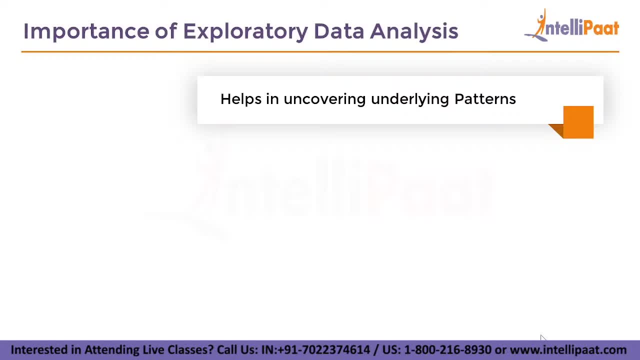 visible by just looking at the data. So let's say, if you are looking at the data, you are looking at the data of a particular country And if you are looking at any data which is related to insurance companies, you might not be able to find the patterns in how the people are paying their premium just by looking. 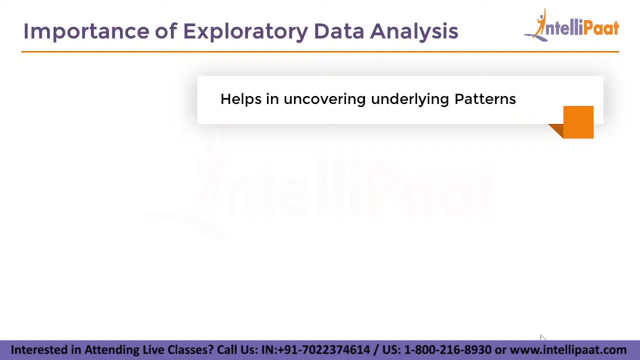 at it And, when it comes to EDA, it will help you identify those patterns and actually work on those insights. Next off, EDA can highlight useful relationships between the data points to gather insights. Now, taking the example of insurance data again, we can actually find out how and why people 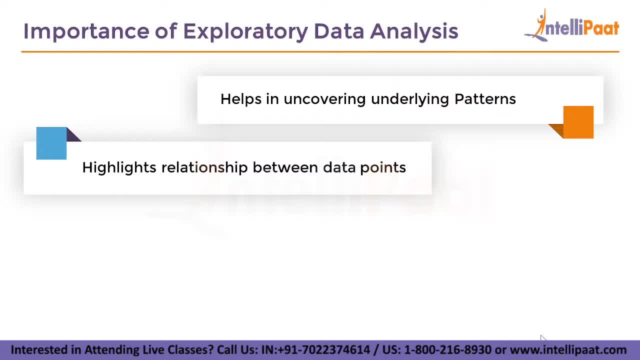 are paying their premiums on time, Or what are the differences Or different parameters which are holding them from paying their premiums on time, etc. EDA also helps in restructuring the data according to the problem statement. Let's say we have to create a prediction model against some data that we have. we have to 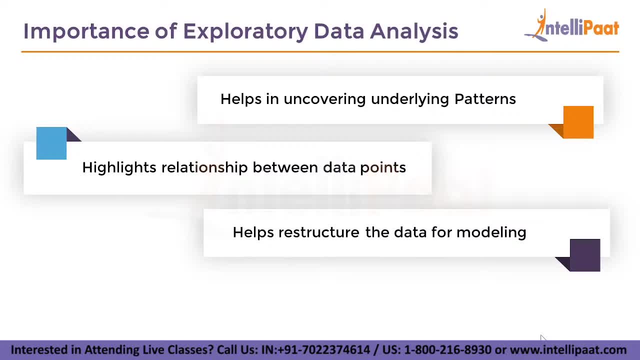 know how we are going to structure that data. Do we need the outliers, Do we need the null values, Or do we actually need to standardize the data for further computations? So that is where EDA comes into the picture. And last but not the least, 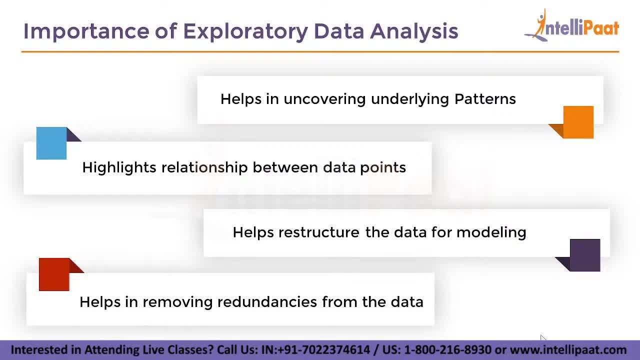 EDA helps in removing the redundancies from the data, which I have already mentioned, the outliers and the data imputation techniques that we are going to use to replace or either remove the null values. Now that we have a clear idea of what exactly EDA is and how, it is very important for us. 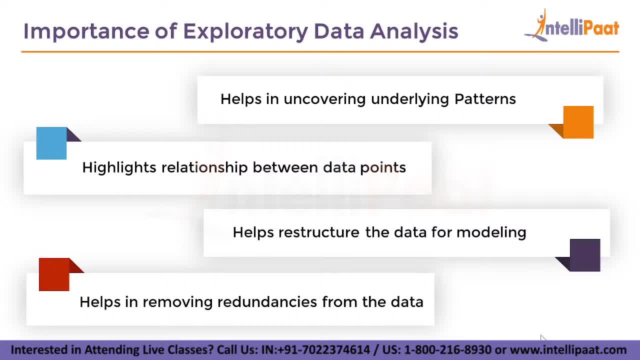 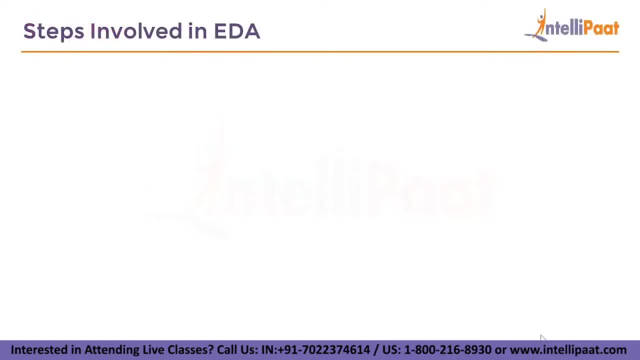 to learn about the exploratory data analysis, let's go ahead and check out the steps involved in the exploratory data analysis. So the steps involved in the EDA starts from how you load the data. So the steps involved in the EDA starts from how you load the data. 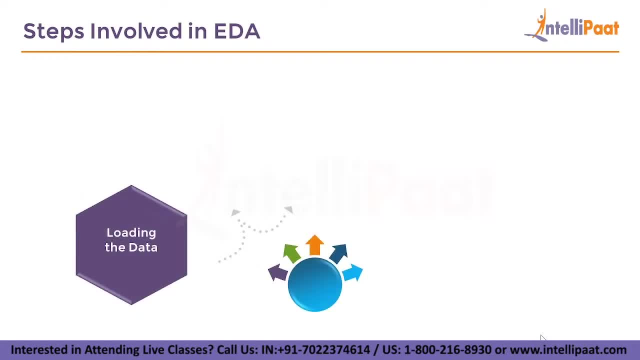 So the steps involved in the EDA starts from how you load the data. So when you load the data into your program, that is where your actual EDA begins, and that is the first step of the entire cycle. also, Once you are done with loading the data, comes the data visualization, where you use the 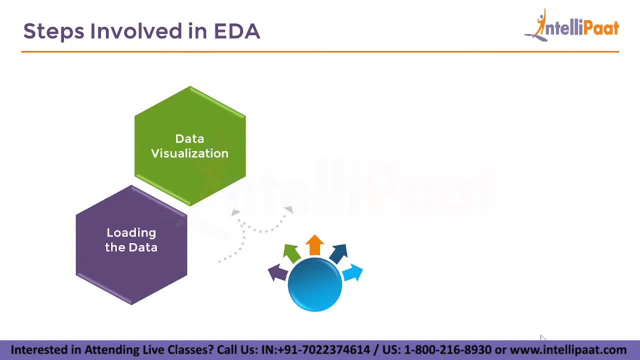 data visualization tools. for example, if you are using Python, we have Matplotlib, we have Seaborn. we can use Plotly to derive different plots from the data which is going to explain the distribution, the piqueness and other important points, like outliers, etc. 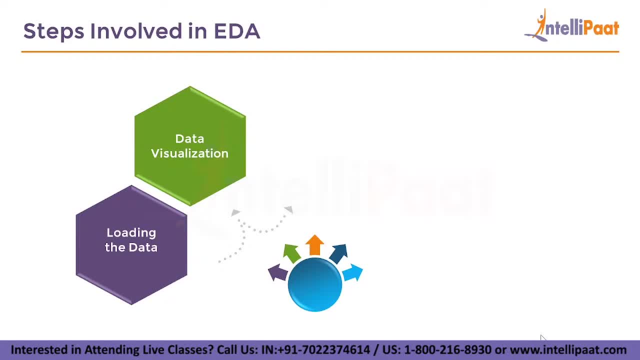 Okay, Then we can also find out the relationship between different variables using data visualization. Next up, the third step, is data imputation, where we are going to figure out how we are going to replace null values or how we are going to deal with them. basically, 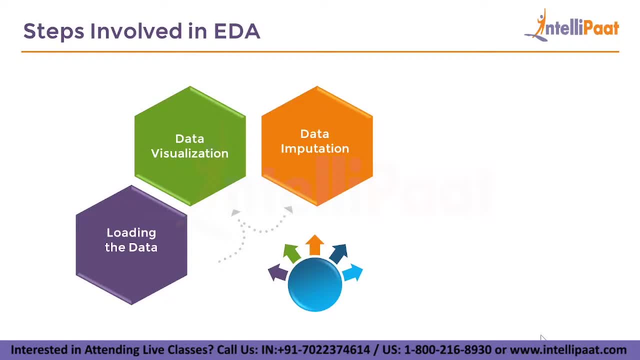 So let's say, if we have a distribution which is a normal distribution, we can just simply replace the values with mean. If we don't have a normal distribution, let's say if it is positively skewed, the distribution, then we can replace the value. 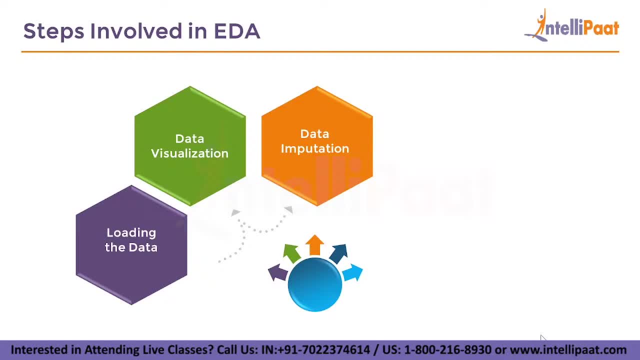 with a median or otherwise. if the presence of null values is very minimum, or let's say less than 5% of the entire data, we can just remove those values or drop those columns. Now, moving on to the next step, that is, the outlier analysis. 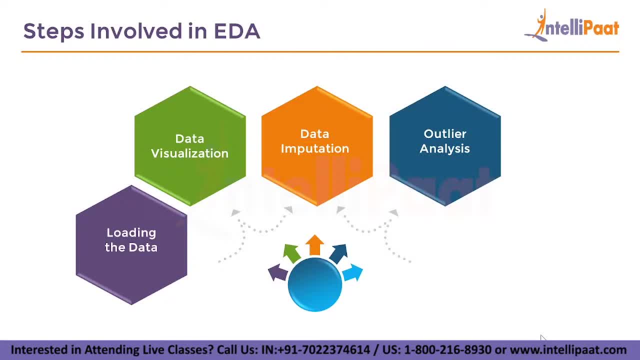 With EDA we are able to do the outlier analysis also. We can identify which features has the outliers and we can also analyze and basically remove those outliers And if we want to keep them, we can take a decision on that as well. 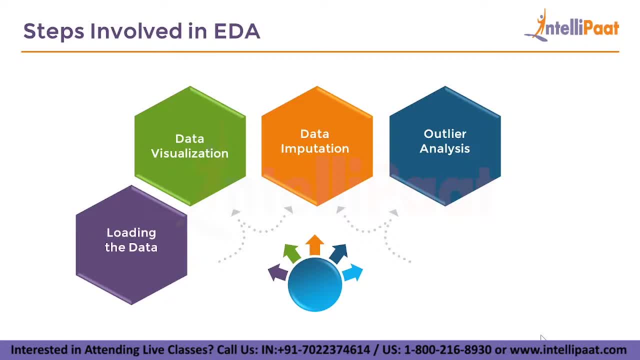 So that is also covered in the EDA. on repeat, So that is also covered in the EDA. And, last but not least, the fifth step is gathering the insights. So, from all these steps that we have performed, we have to come to a conclusion that our data has several insights. 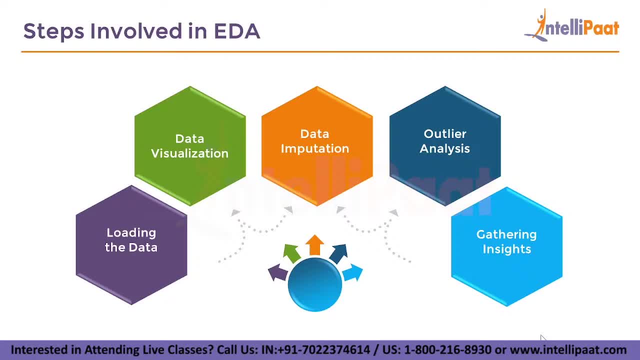 For example, let's say, if I am analyzing the IPL data like we have done in one of the previous sessions, what we have done is basically carrying out an entire EDA on that particular data and we have found out the 10 best players of that. 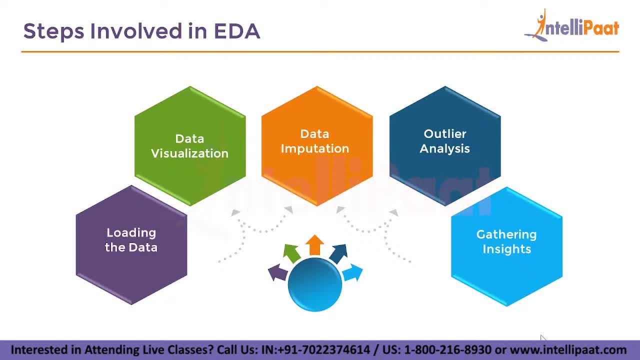 repeat, we have found out the 10 best players from that entire data. So, similarly, we have to gather insights from the data. and now that we have actually understood the steps involved, we have understood the importance and the basic definition of EDA. let's move on to. 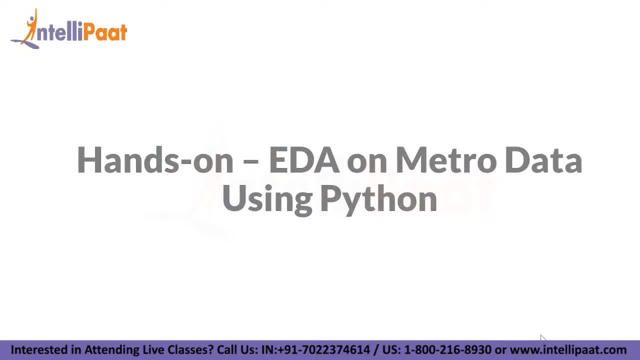 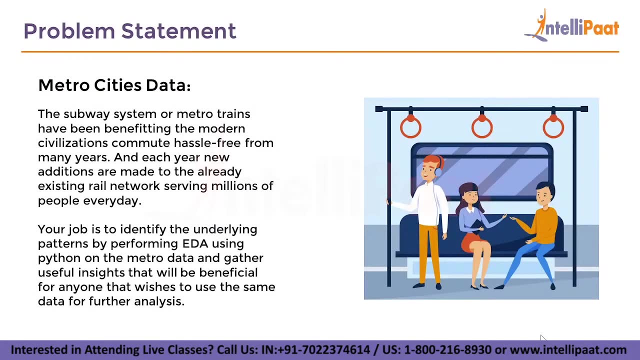 the hands-on part where we are going to perform the EDA on metro data using Python. Before that, let's just quickly take a look at the problem statement. So we have the metro cities data and we And we already know that subway system or the metro trains that we have in the various 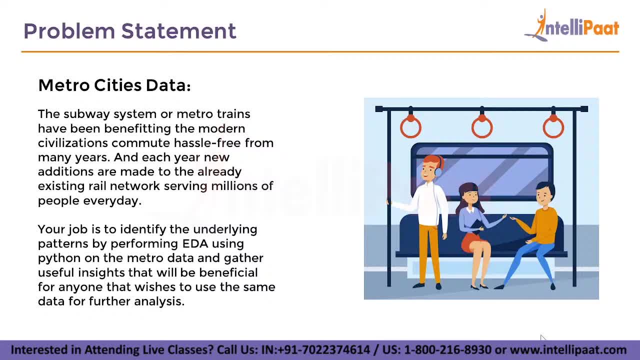 countries, has been there for civilizations and has been helping the modern civilization to commute in everyday life, And it is a very big network all around the world. So we have gathered that data and our job is to identify the underlying patterns by performing EDA, where we are going to use Python on the metro data. 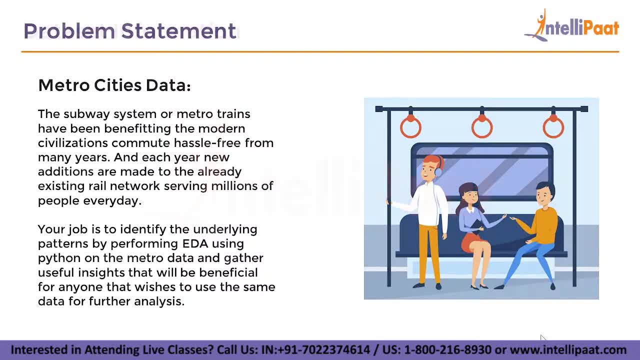 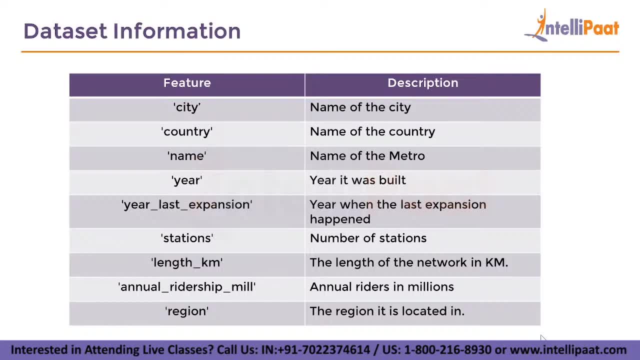 And in the end, we are going to gather a few insights from the data. So let's also take a look at the data set, how we have all these features: city, country, name, year, year, last expansion stations, length, kilometer, annual ridership mill. 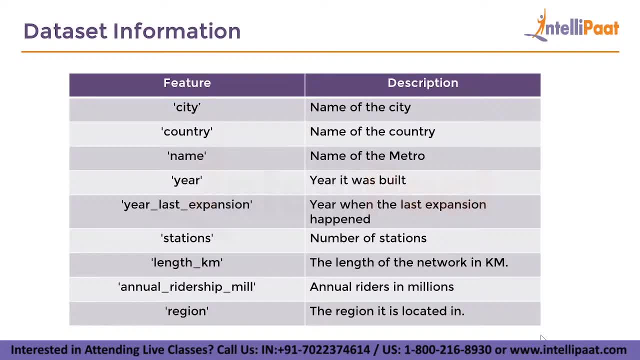 and region. So we have also described the columns here. So city is basically the name of the city. then we have the name of the country, the name of the metro, the year it was built and the year when the last expansion happened for that particular metro. 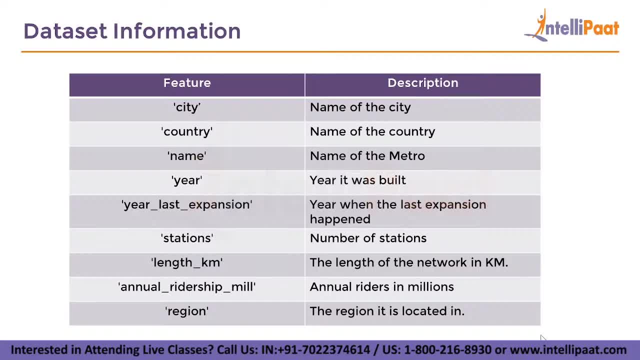 And then we have the number of stations, the length of the entire network In kilometers, and then we have the annual riders, which is in millions, And, last but not least, we have the column with region, which is basically nothing but the region where it is located in. 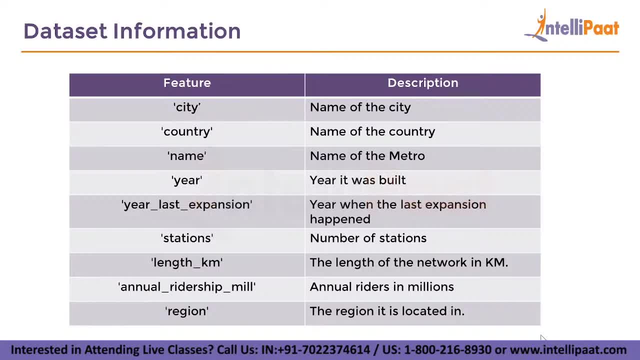 It could be North America, it can be Europe, it can be Asia, or it could be Australia, And then we have Latin America as well. So we'll quickly go to the notebook and perform EDA. So let's get started, guys. 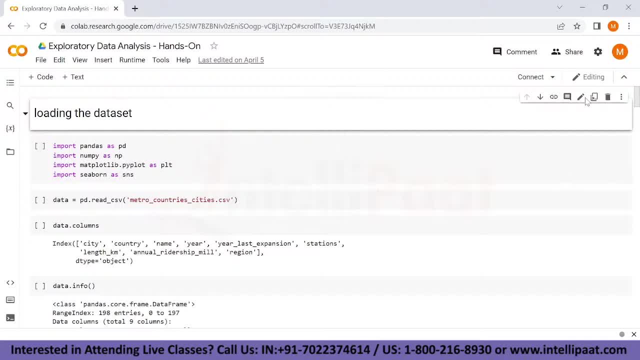 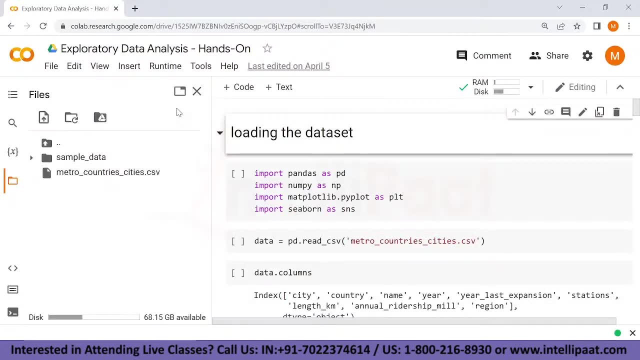 All right. So this is our notebook that we have created. Increase the visibility here. So, as you can see, we have already imported the dataset and we are using the Google Colab for this. You can perform the same on Jupyter Notebook, if you like. 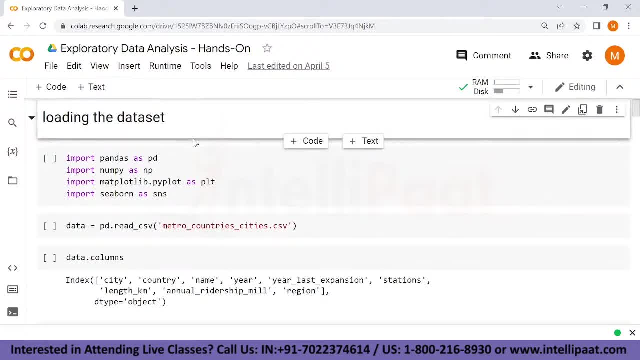 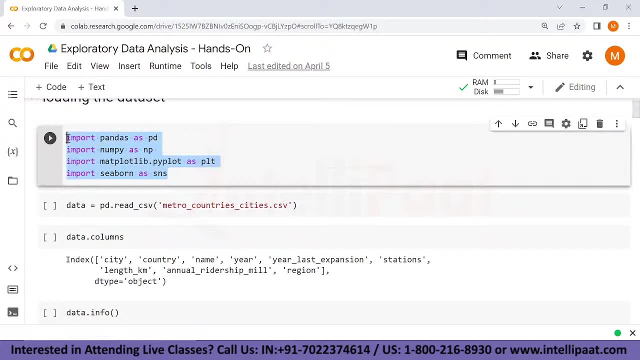 It's up to you guys whatever suits you better. So we are going to be performing EDA using Google Colab. So first of all we have to load the dataset and we have imported all these libraries, Pandas, because we are going to be using DataFrames here: NumPy for basic, few computations. 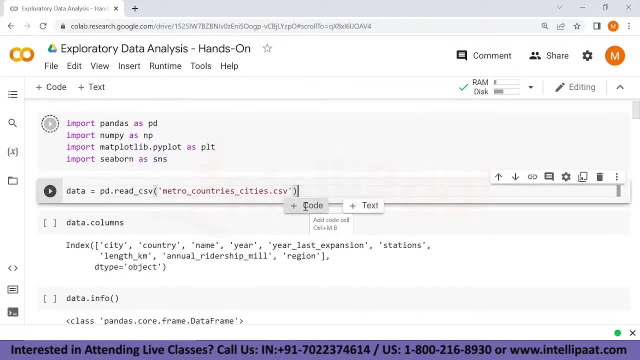 Matplotlib and Seaborn for visualization. So loading the data is very simple. guys, We can use the readcsv function over here from Pandas module and with the file name. If you're using Jupyter Notebook, you might have to get the directory over here and you. 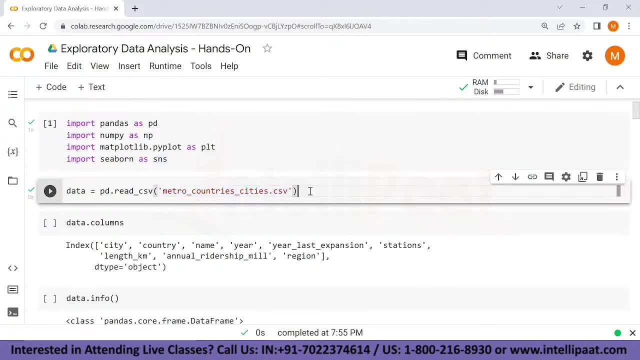 may find out that you're facing a few errors importing the data. But don't worry guys, You can reach out to Intellipaat and we'll be happy to help you with this problem. And then with this, we are basically done loading the data. 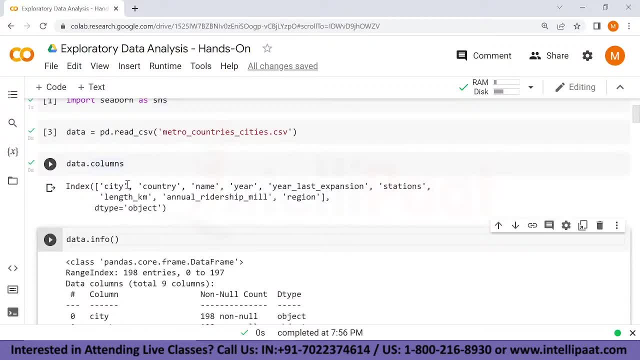 So the very first step that I'm doing over here is getting the name of the columns, And then we're going to load the data. So the very first step that I'm doing over here is getting the name of the columns. So the very first step that I'm doing over here is getting the name of the columns. 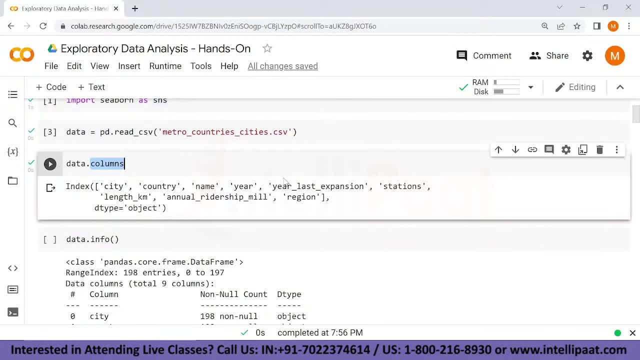 So the very first step that I'm doing over here is getting the name of the columns. So datacolumns give me the column names. So we have city, country name, year, year, last expansion that we have discussed while discussing the description of all these columns in our data. 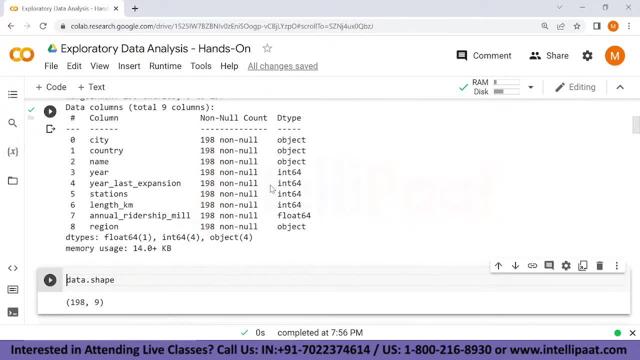 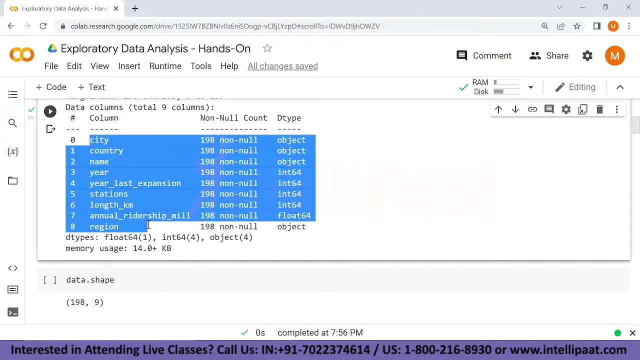 Next up we have datainfo. So info is going to give me the information about. as you can see, we have three columns here. One is having the column name, basically all these names. Then we have the number of values and how many of them are non-null. 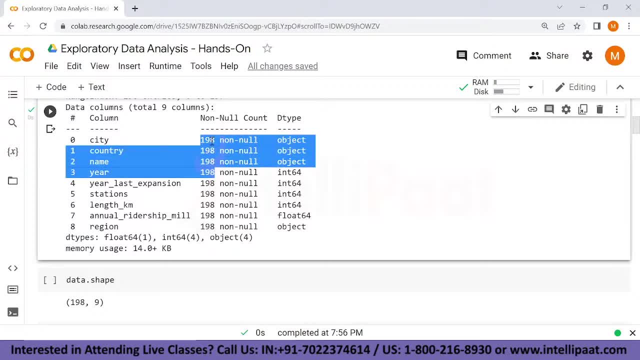 As you can see, we have 188,. repeat, As you can see, we have 198.. We have 198 values over here which are all non-null. The data type here is object for three columns. Then we have integer. 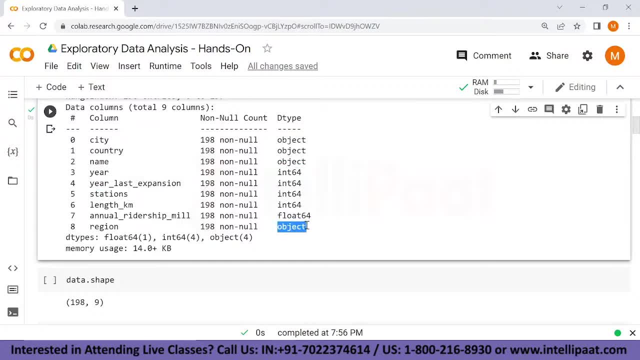 The annual ridership is in float And then we have object again, So we might have to change these data types. if we are going to perform some linear regression, let's say So that comes after we have gathered the insight or before we are preparing our data for the 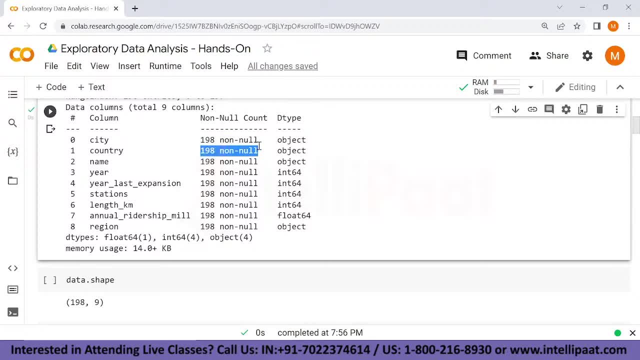 modeling. So that is also one of the things that we can cover in the ADA, where we look at all these data types And figure out which one needs to be converted to, let's say, integer. Now let's go ahead and check the shape of the data with datashape. 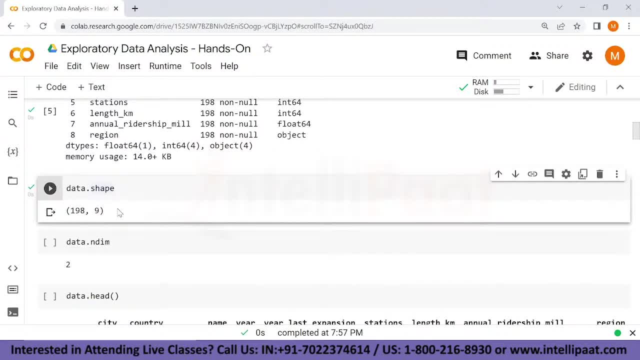 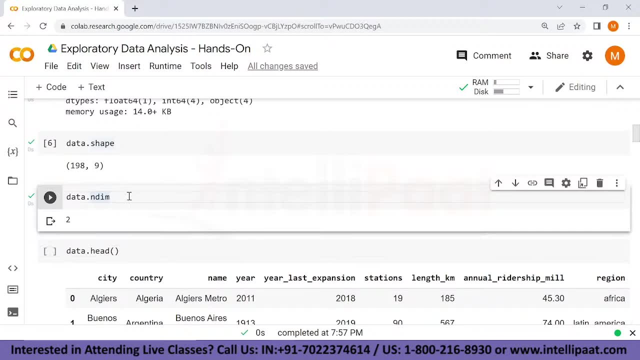 So we can see we have 198 by 9 is the shape of our data over here. We can check the dimensions also. So checking the dimensions helps you when you are performing. let's say you have a data which has 64 dimensions. 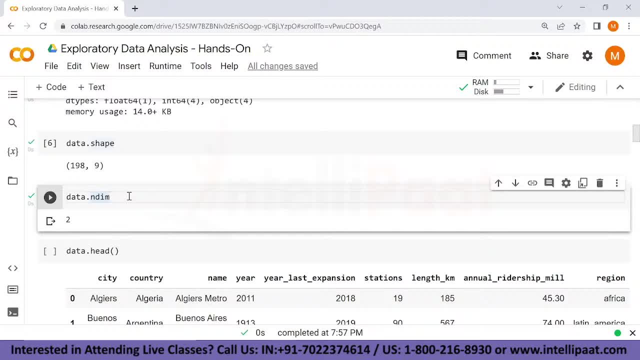 Then you may have to perform dimensionality reduction over there, which will help you in preparing your data for the modeling, And that is why we are going to check the dimensions, And that is why checking the dimensions is also one of the good practices when you are. 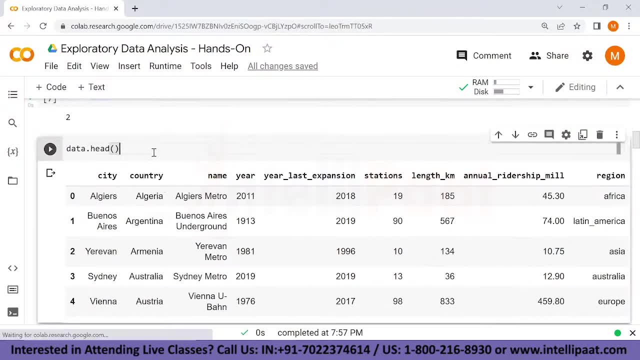 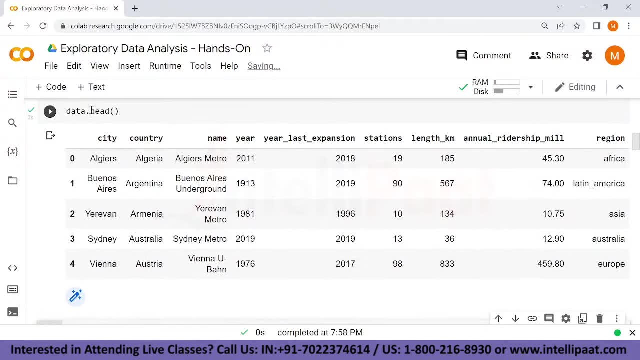 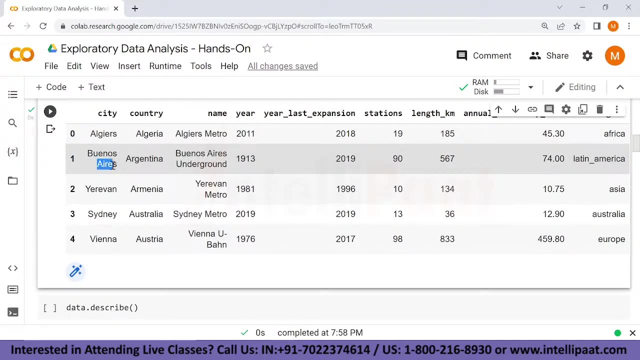 doing EDA, All right. So this is the part where we describe our data. So, first of all, what we are doing is we are getting the first five rows in our data set using the datahead method over here, As you can see, the first five rows in our data. we have the cities, we have the country. 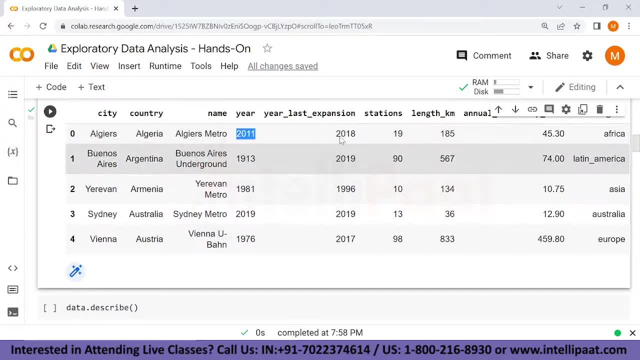 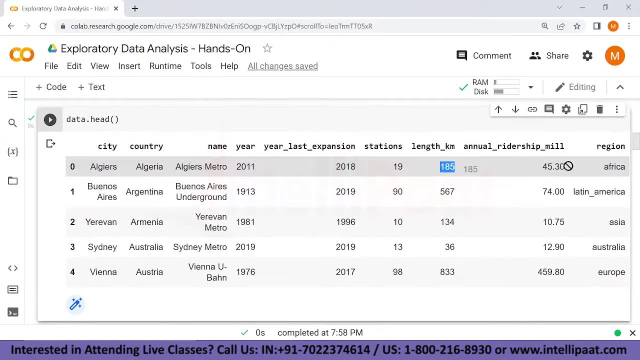 the name of the metro, the year it was built, the last time it was expanded, And we have the city, And we have the country, And then we have the stations: the length in kilometers, annual ridership in million, and then Africa. 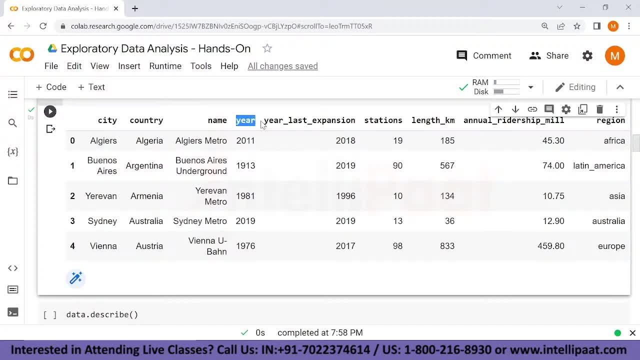 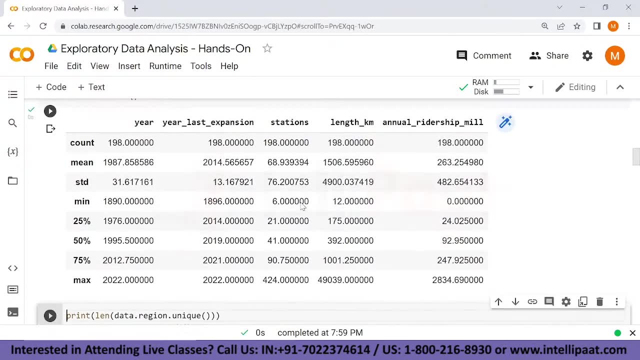 So we have a lot of variables here which are not integer or float type. So what we are doing is we will describe the data, but we are not going to get the values for those particular columns. like, if you can see over here, the describe method does not. 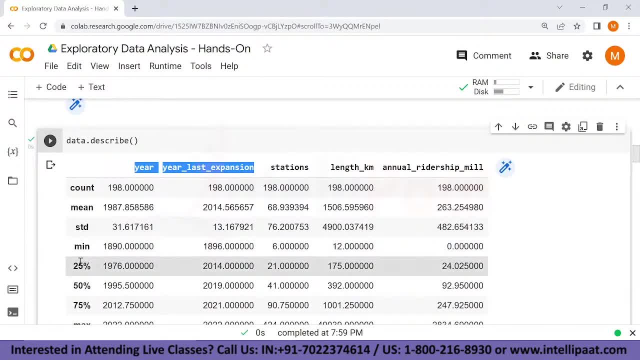 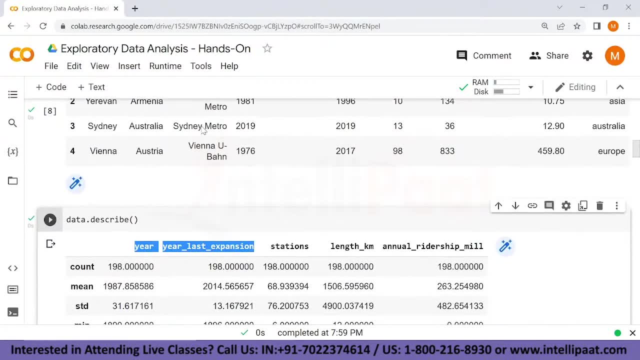 fetch us the count mean standard minimum: 25 percentile, 50 percentile, 75 percentile and so on. For the columns city country, we don't have name over there, we won't be having regional as well. 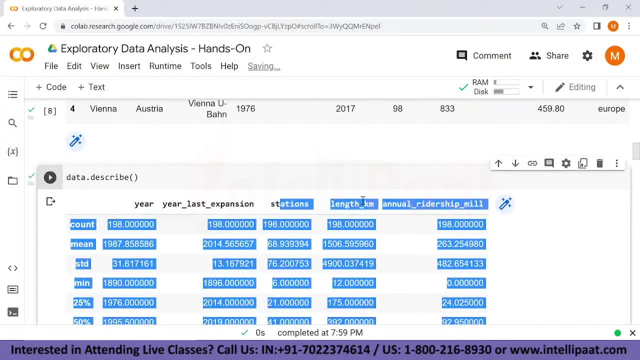 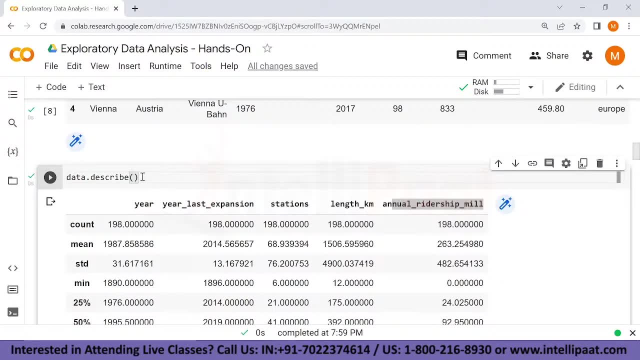 So we have only got the year year last, expansion, the stations, length, kilometer and annual ridership. So this is one pointer that you can make a note of. Whenever you are using the describe method, it is not going to get you the values which 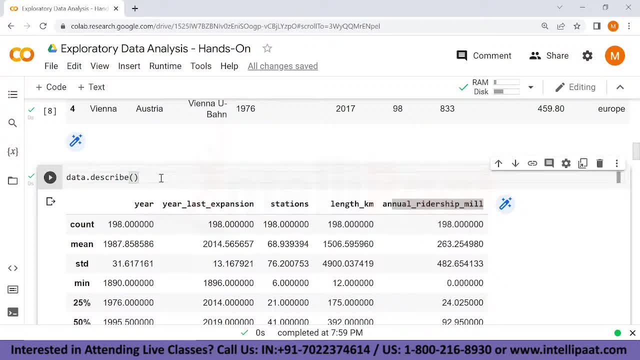 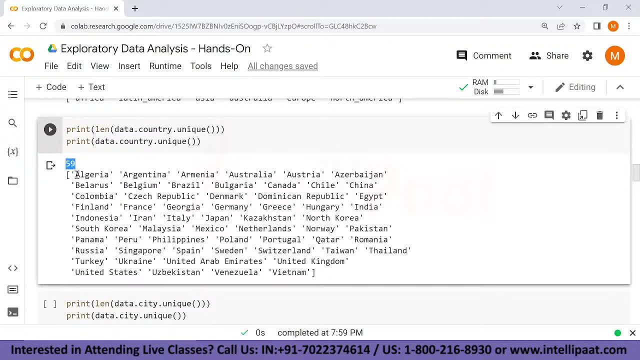 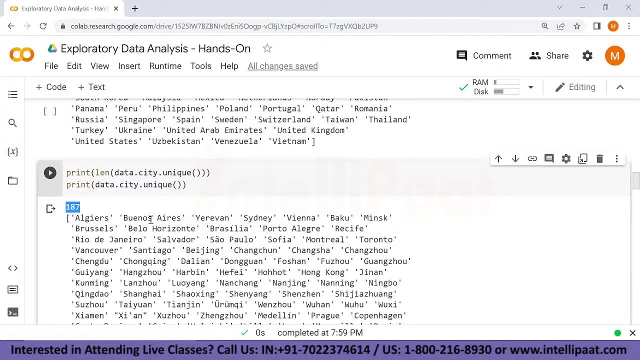 So we provide the metro network in our data and these are the country names, And then again, if you do that for the cities, so 187 countries from the world In our data has the metro networks or metro trains. so this is a very simple finding from our data. 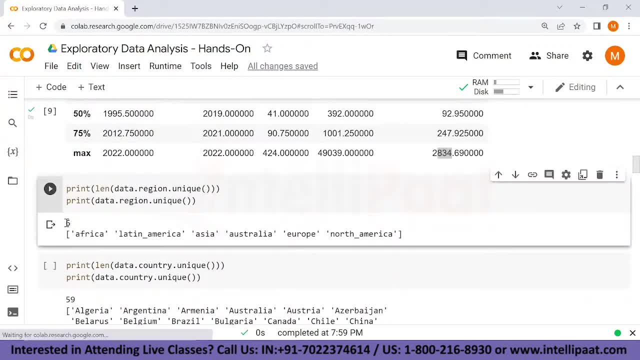 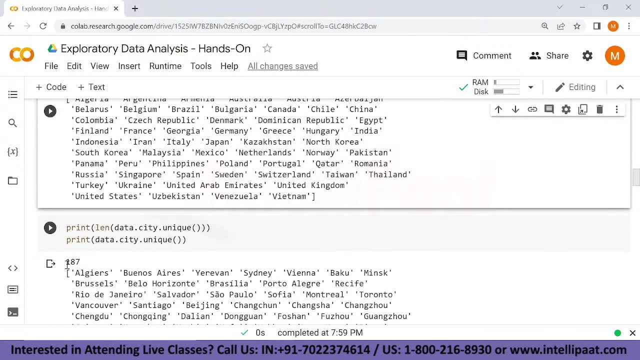 As you can say, in these 6 regions, 59 countries have metro stations and out of this 59 countries, 187 cities are there. So there are eight regions. So that is our image information. So that is our image information. 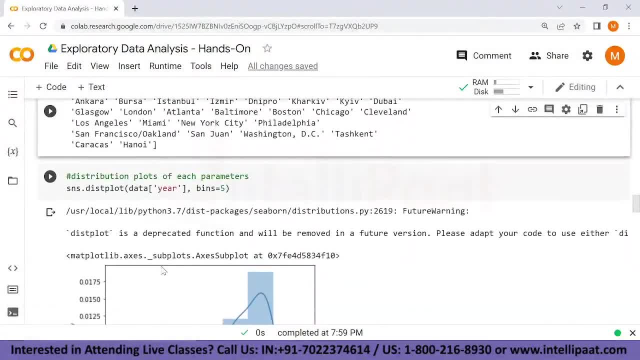 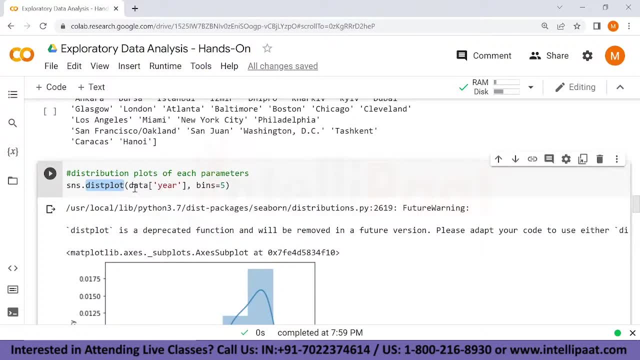 initial finding from the data. Now, when we move on, let's check the distribution plots for each parameters. Now we are using CBON over here to create a distribution plot. Now distribution plot will tell you a lot about your data. Basically, it will give you if. 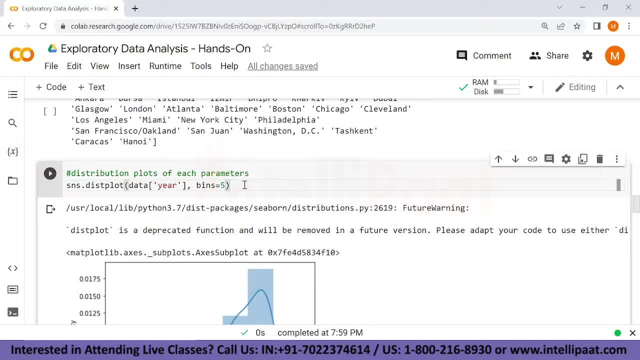 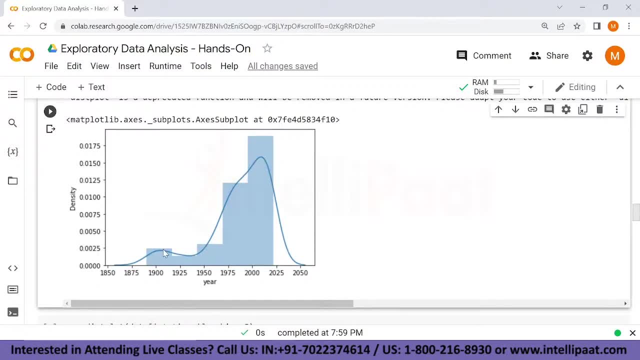 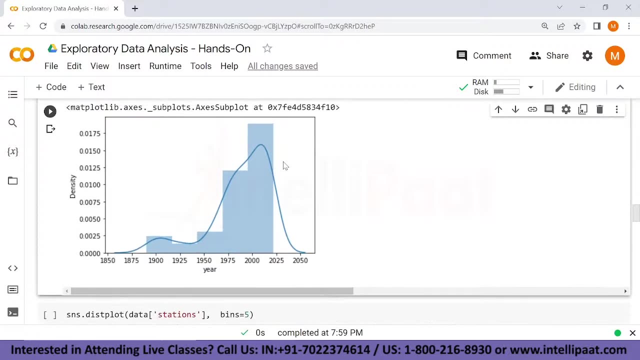 it's a normal distribution or if it is positively skewed or negatively skewed. So if we take a look at this data, this is negatively skewed because we have a lot of values towards the end of the distribution, And that is how we can estimate or basically interpret this. 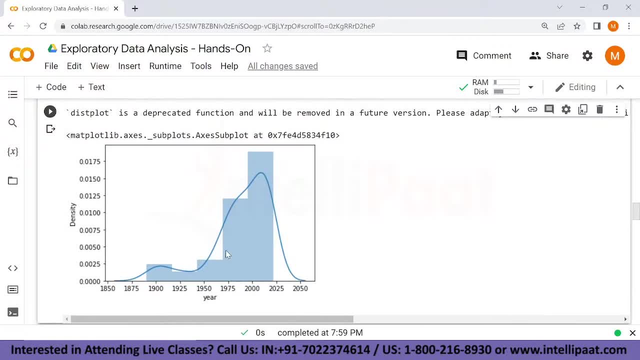 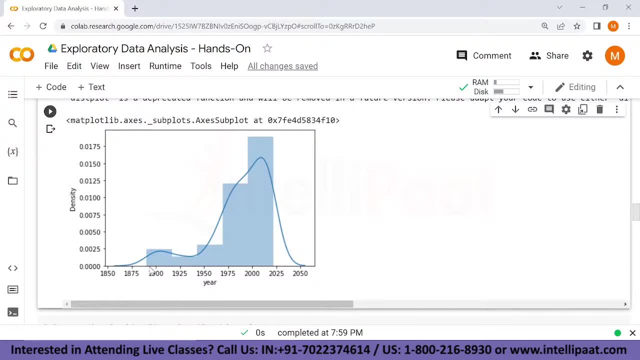 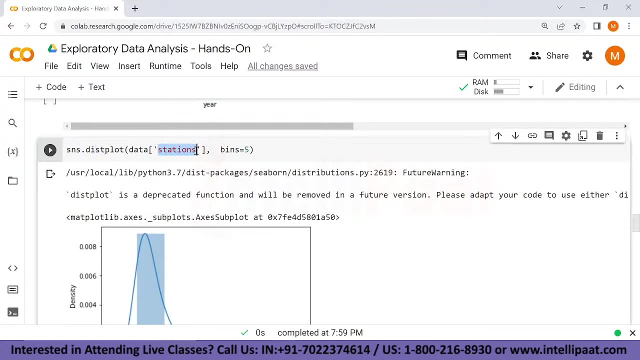 data. So most of the metros were built after 1975, we can assume that- And the first ones were built somewhere around 1900s or before that, in very less numbers. When we take a look at the next plot, which is about the stations, this is also skewed data, not a. 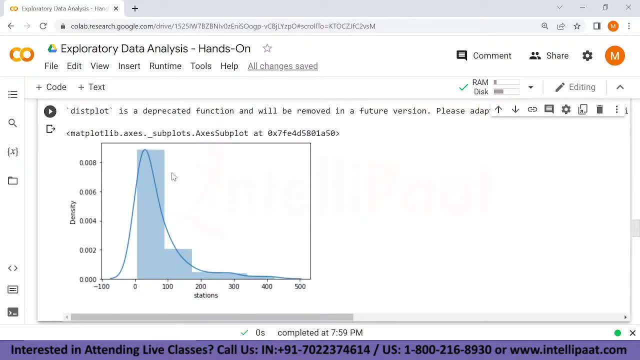 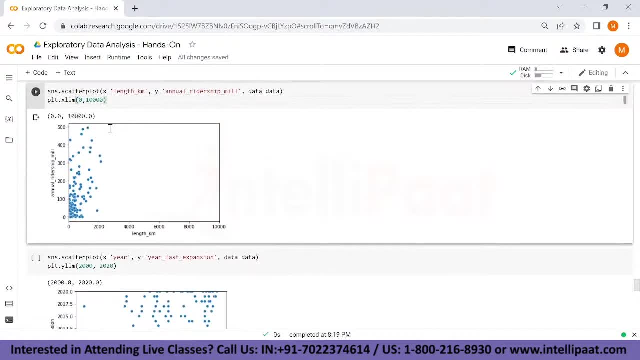 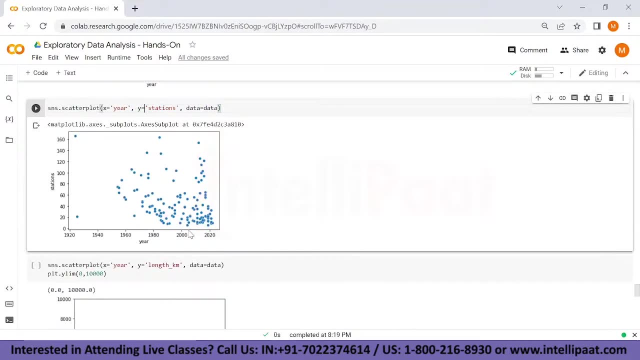 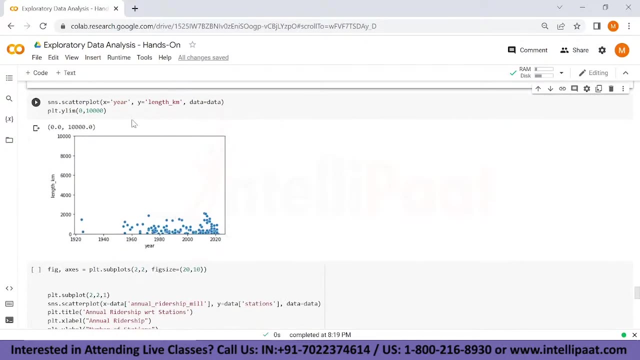 Similarly for x limit. also we have taken that for length in kilometers, and when we check for year end stations this also does not show a considerable amount of relationship. So this does not actually show a very good relationship between the two. For year end length kilometers, also there we can't find any considerable amount of relationship. 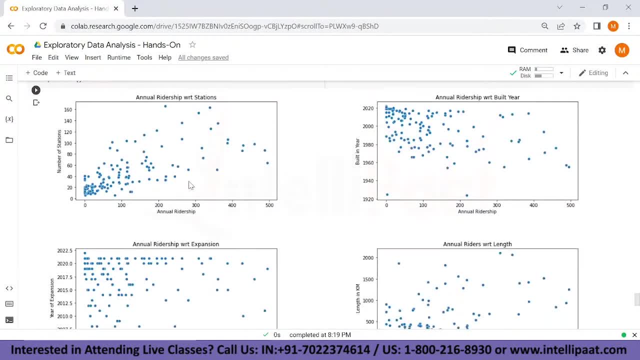 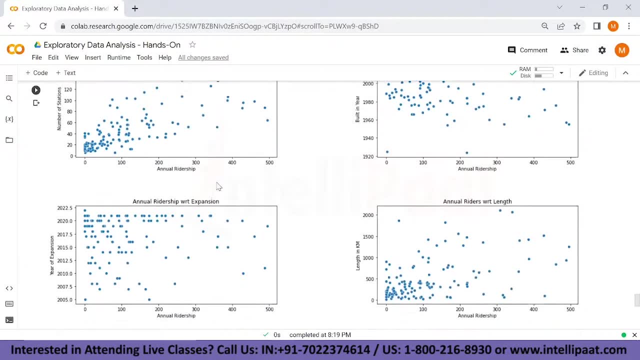 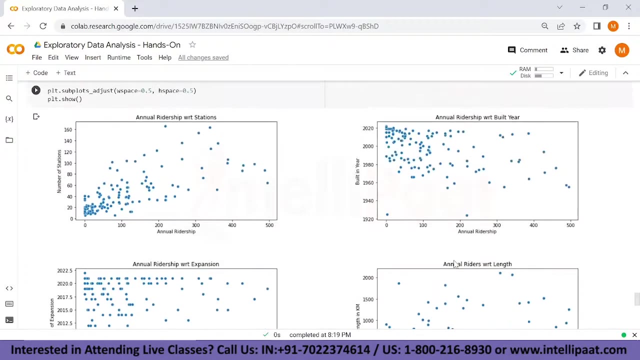 and then again, if we plot all these subplots, these are the subplots that you can get- and annual ridership with respect to build tier, annual ridership with respect to stations, annual ridership with respect to expansion and length. So length shows somewhat linear relationship and the number of stations also show. 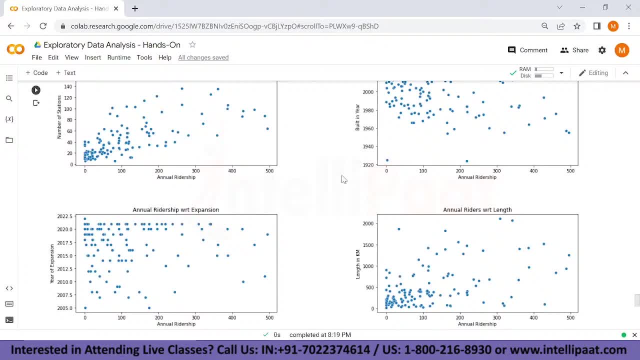 So these two variables or these two features in the data are going to be very useful for us if we go for a linear regression model, let's say. So these two will be able to decide how our data looks like and how we can actually predict some of these values. 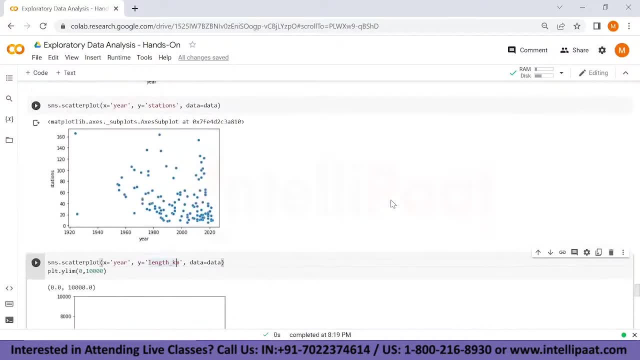 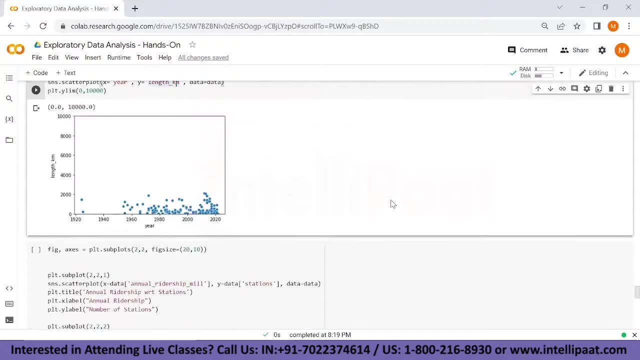 Since we have not used any of the object columns. if we do a little bit of hot encoding or label encoding on that, we might be able to find out relationship over there as well. So you can take that up as an exercise. so I will tell you two questions you can solve. 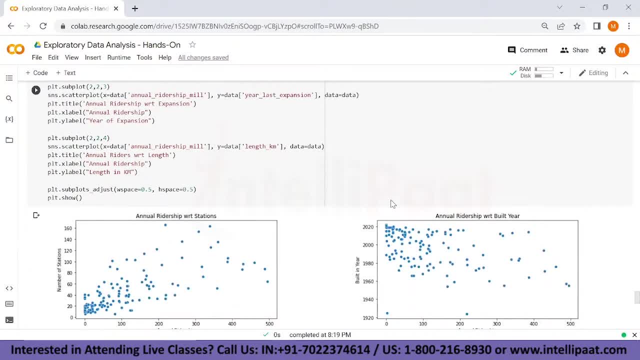 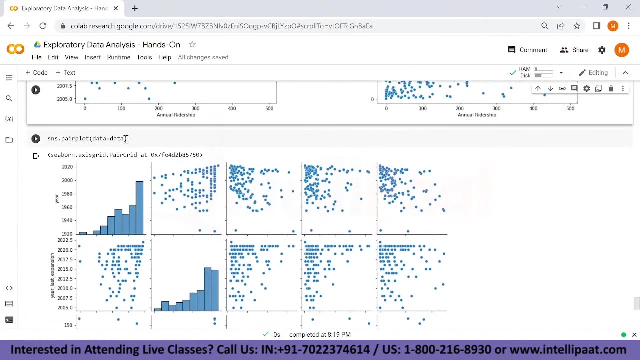 Convert the object data type in this particular data into an integer data type or perform label encoding in that, and find out the relationship between those variables and the annual ridership column. So this is one exercise you can take from this session and then again if you just want. 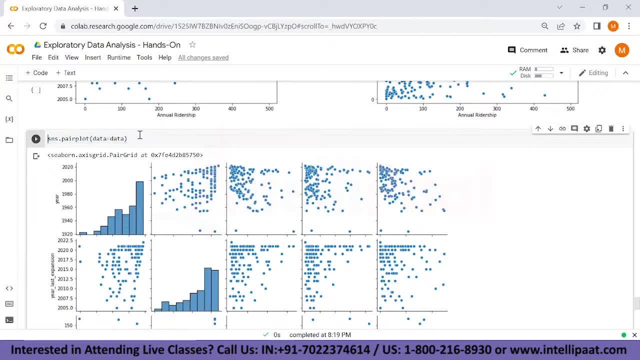 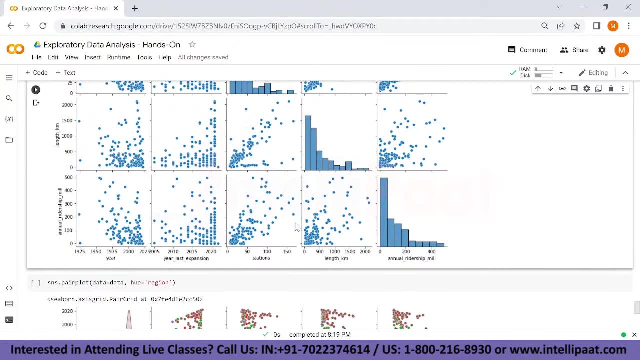 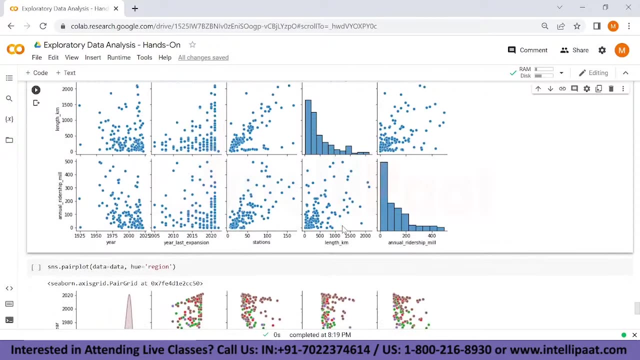 to get the relationship easily, you can just use the pair plot, which gives you all these plots with respect to each of the columns and with the annual ridership in millions. we can see two columns that are showing considerable amount of linear relationship and we are going to conclude with that. 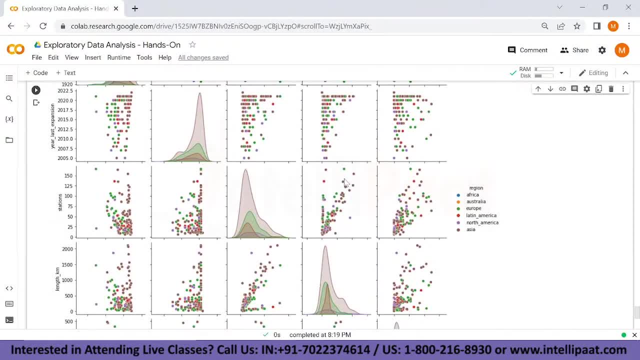 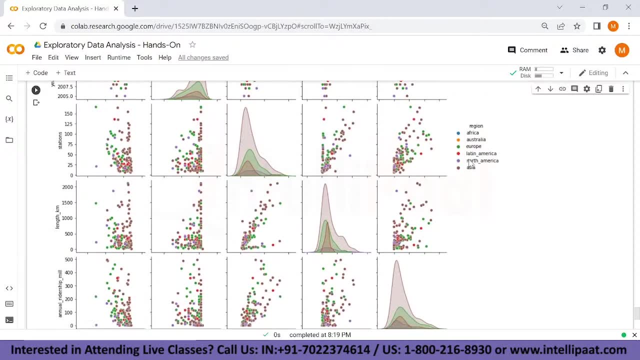 We can add the hue as region also, where blue is Africa, Then we have the color, We can add the color, We can add the color. We have orange, which is Australia, Europe in green, Latin America in red, North America and Asia. 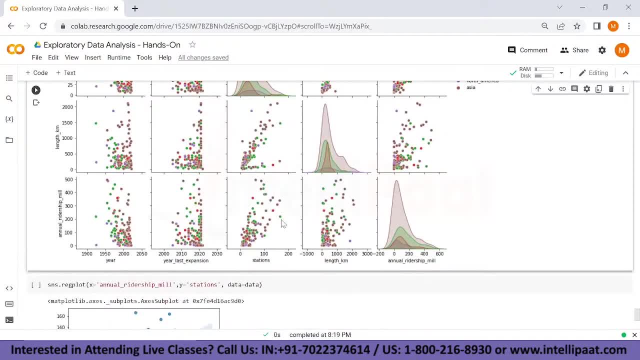 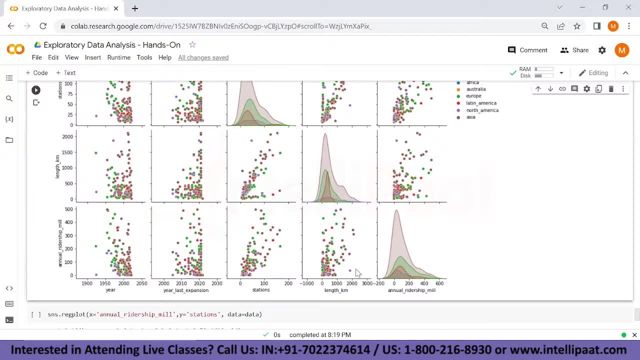 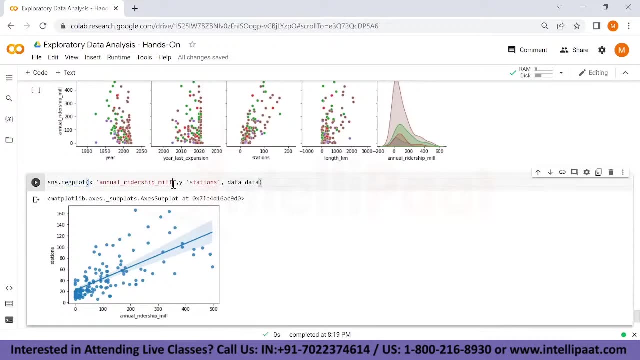 So if we check over there, the extremes are on Europe. over here, number of stations And length in kilometer is in North America. the extreme. That is how we can visualize the data guys to gather insights and also create a regression plot. so annual ridership and the two columns that we have gathered which are stations, the 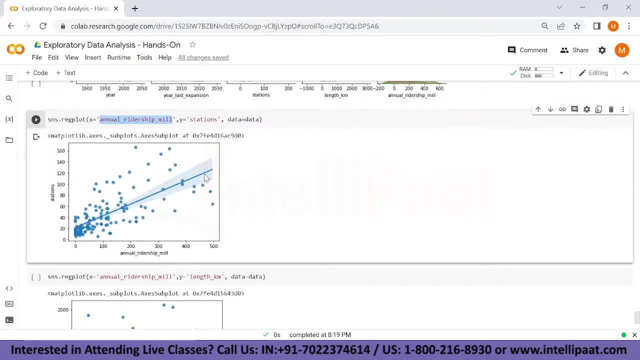 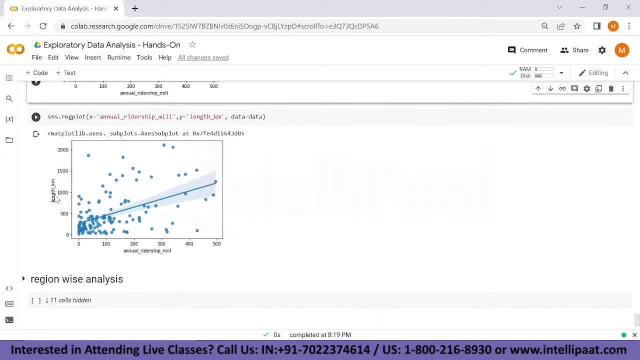 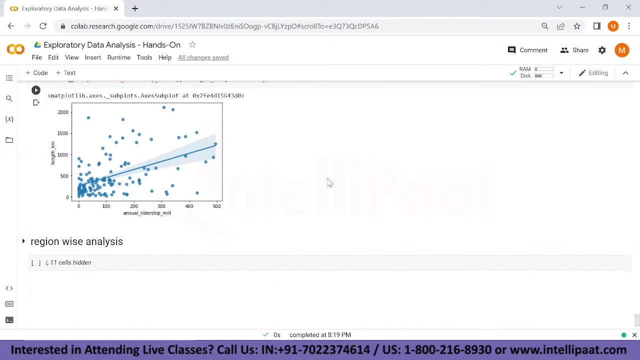 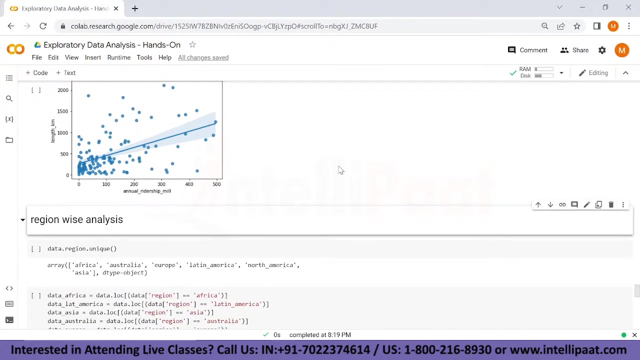 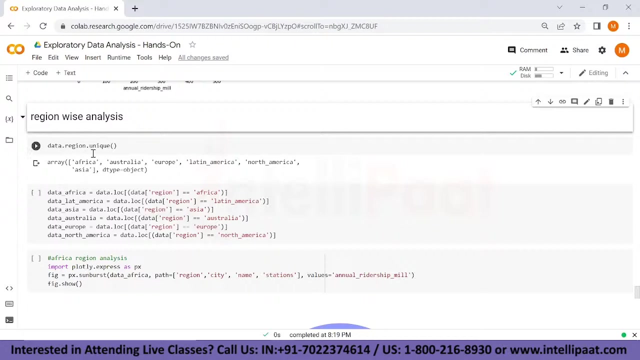 best fit line is over there, and here the error we can reduce. and same again if we plot this for annual ridership in million width, length in kilometers. so that is how we plot the regression line also. now, to sum up this session, let's also do a little bit of region wise analysis and also a little surprise for you where we have used a few pi plots using plotly. so that is something that looks interesting and gives you a better picture of the entire data. all right, so 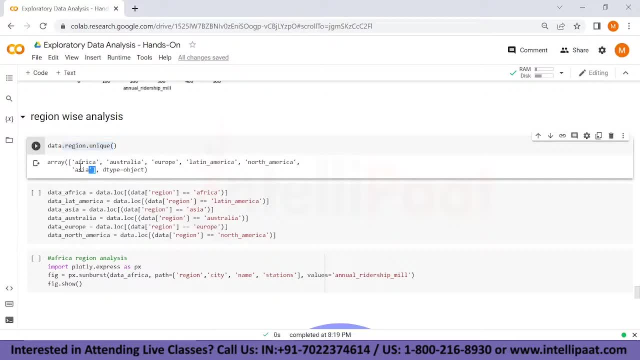 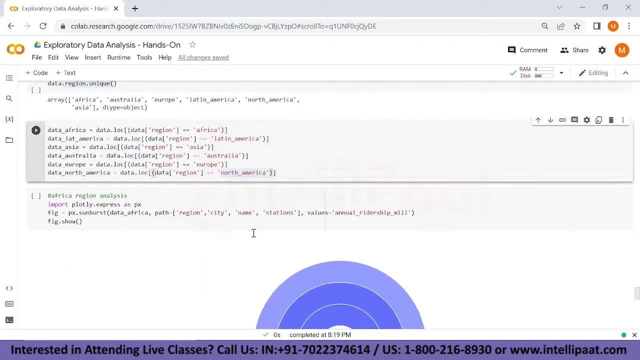 we get the unique values, which is all these six regions. we segregate the data based on all these regions. we're using the data dot, loc or lock where the region is equal to africa, latin america, asia, australia, europe and north america. now what we're doing is we're using plotly for sunburst, which 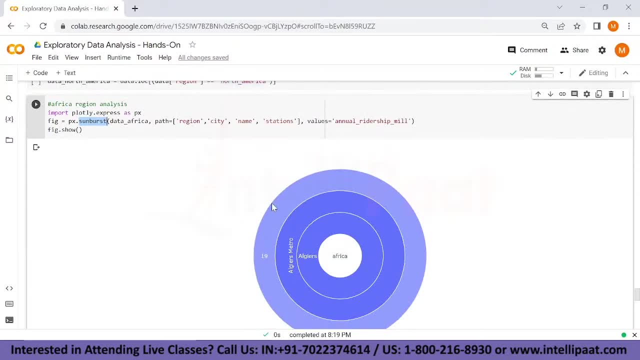 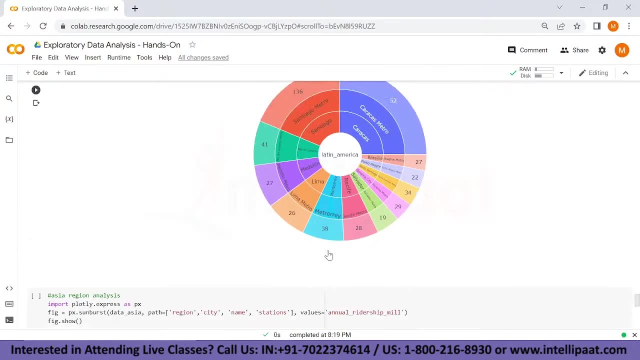 looks like a pi plot, but it actually opens up when you, when you click on these. all right, so just to quickly give you a review on this. we'll go to the asian and late. okay, let's check for latin america first. so this is a sunburst which. 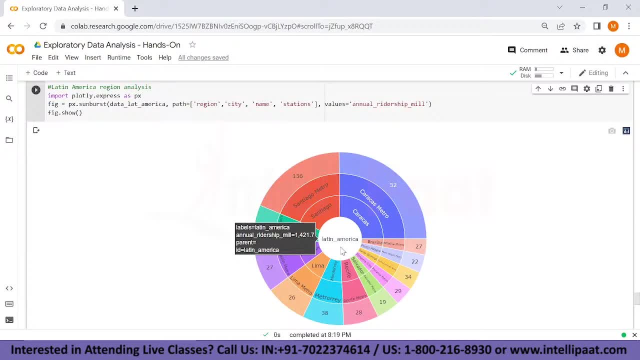 is going to give us the clear picture of the entire data or the entire metro network in the latin america. what? what we have is all these countries. so these are countries. let's say, all right, i'm sorry guys, these are not the countries, so we have only used the region. 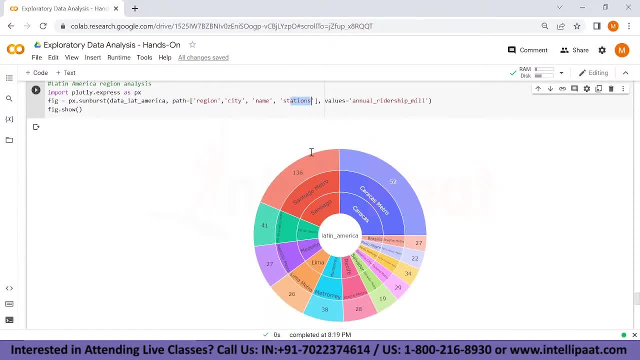 the city name and stations. we have not used the countries. i'm sorry, guys, these are not the countries. so if i click on caracas, we have the caracas metro and which has 52 stations and the million repeat and the annual ridership in million is 358. let's go back, let's check for medellin, and we have the medellin metro. 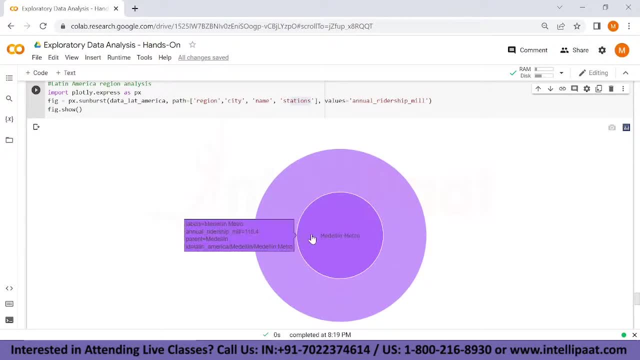 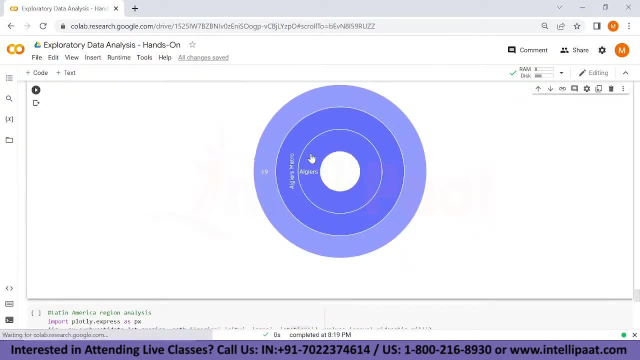 which has 27 stations and the ridership in million is 115.. so i can check that for every city that we have in latin america or in africa, for for in africa we have only one city, alger's metro, which has 19 stations and 45.3 million annual ridership. so this quickly summarized. 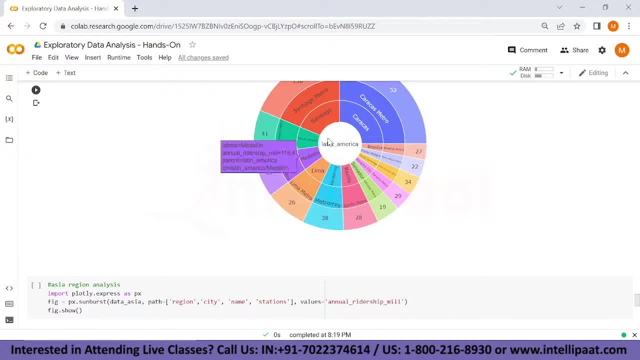 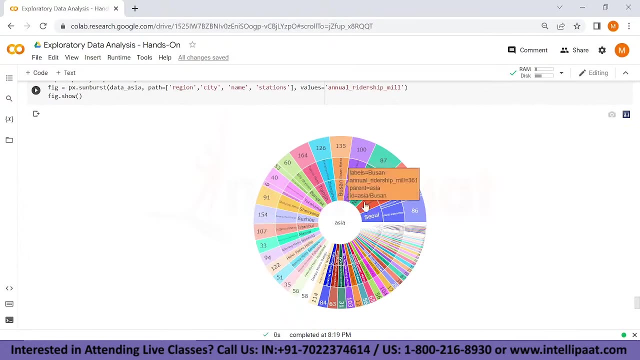 all the data based on regions. so that is how i have segregated the data. if we take- take a look at rio de janeiro, we have the rio de janeiro metro, which has 41 stations, and the annual ridership is 118.7. now, when we have a lot of cities, we have a lot of these columns. so what? 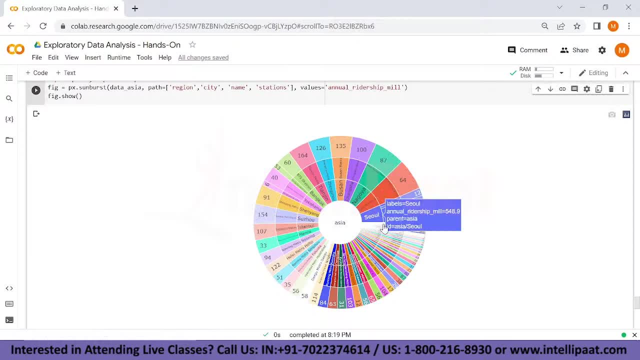 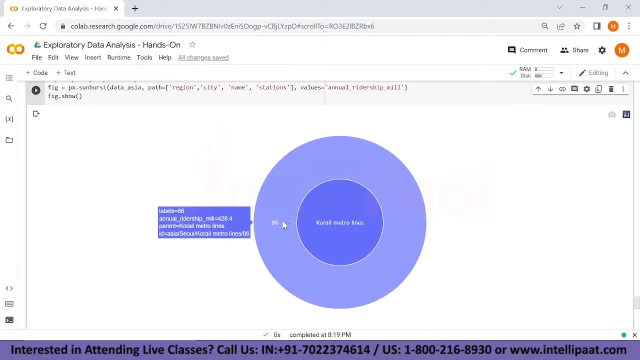 we can do is we just check for the number of stations over here. let's say we have a lot of cities. we go to seoul. seoul has two metros. we have the corel metro lines, which has 86 stations and 426.4 ridership in millions, and then we have the shimbudang line, neutrons, which has 12 stations. 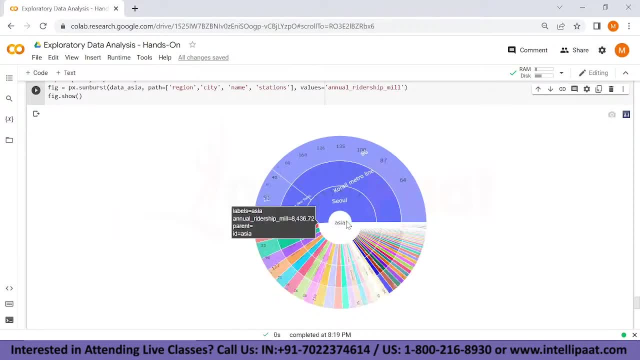 and 122.5 ridership in millions. then in asia we can check for other cities. okay, let's, let's go to istanbul, so we have the istanbul metro stations. they might be. uh, there's manila over there, which has the manila light train system. 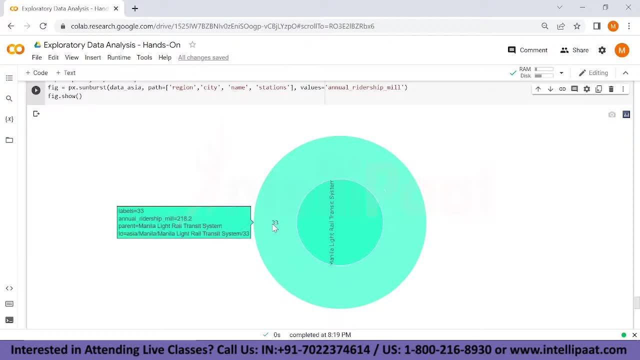 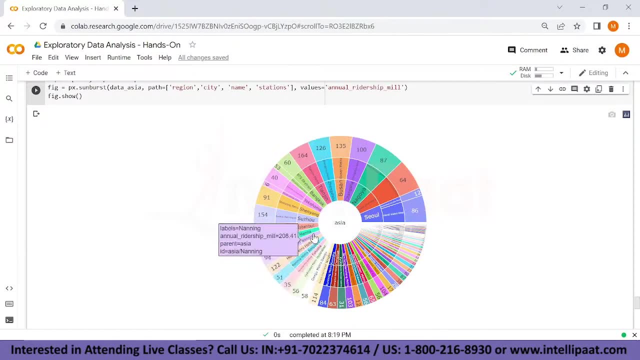 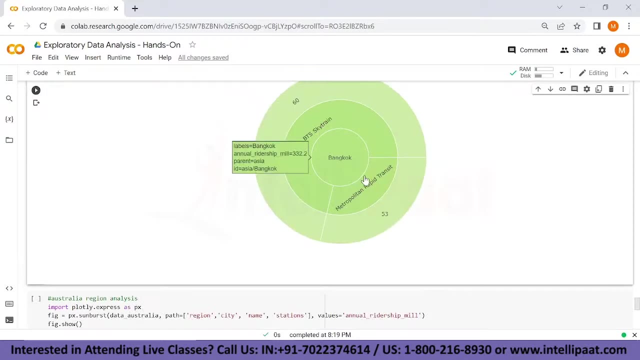 repeat, the manila light rail transit system and number of stations is 33 and 218.2 million ridership. all right, guys. so that is all about how we can create a sunburst. so in bangkok we have bts, sky train, the metropolitan rapid transit, 53 and 60. 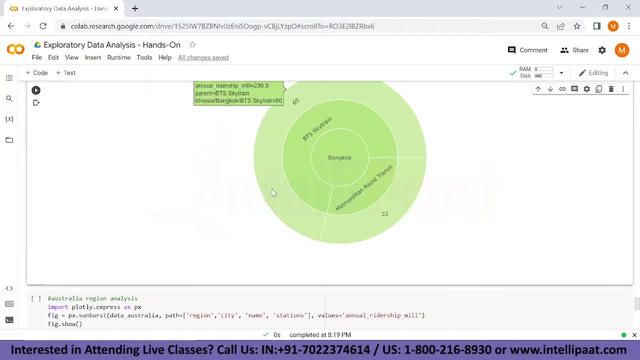 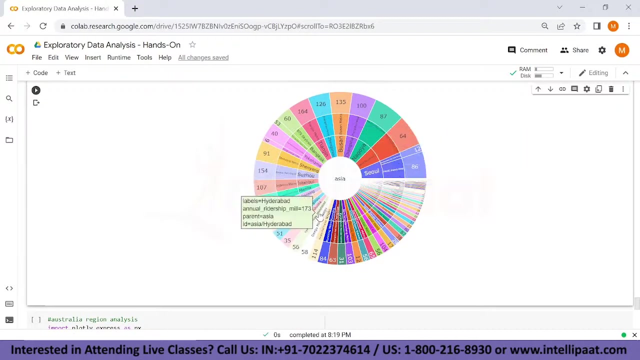 stations, annual ridership 236.9 and 95.3. so we have bengaluru also, which is nama metro, with 51 stations and 174.2 million riders or commuters every year. we have hyderabad metro also, which has 56 stations. 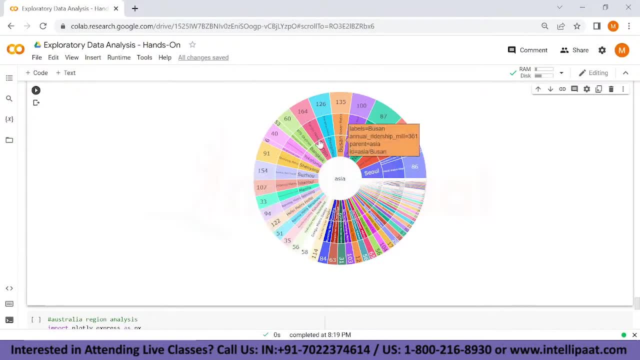 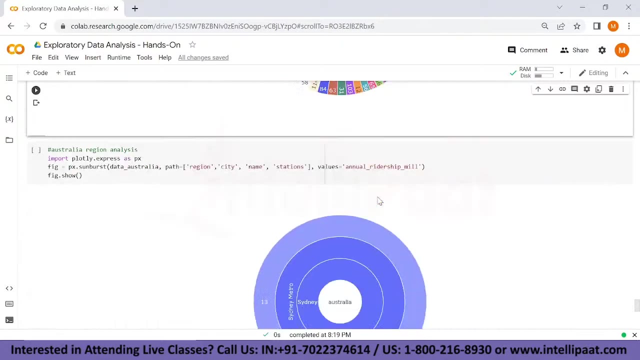 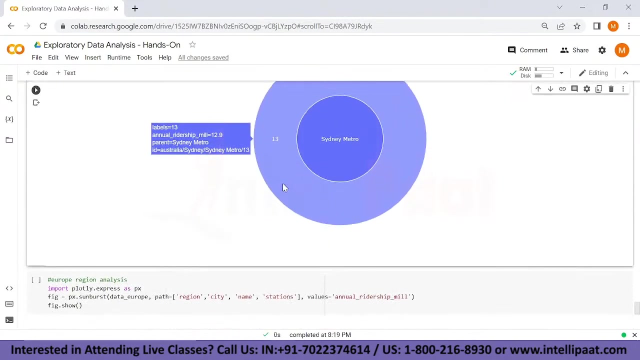 and these are all the summary of all the cities that has metro in the asian region. saint peterborough is also there. the saint peterborough's metro: 64 stations and 495 million. so that basically gives me a summary. then we have for australia with sydney metro has 13 stations and 12.9 million users. and then we have for europe: 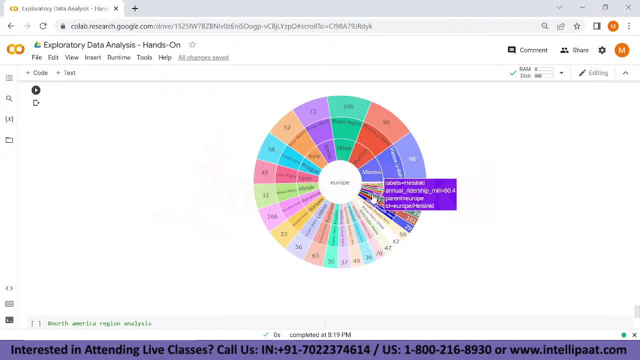 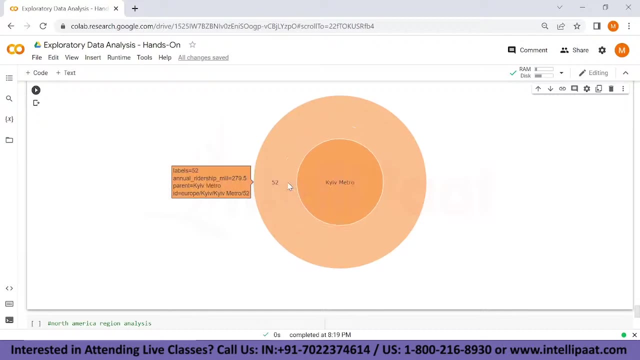 milan, munich, vienna, all these values lisbon, warsaw, minsk, and we have prague, kiv, rome. so for key, we have the kiv metro, which has 52 stations and 279.5 million riders every year. we have for lisbon, the lisbon metro, 56 stations and 184.6 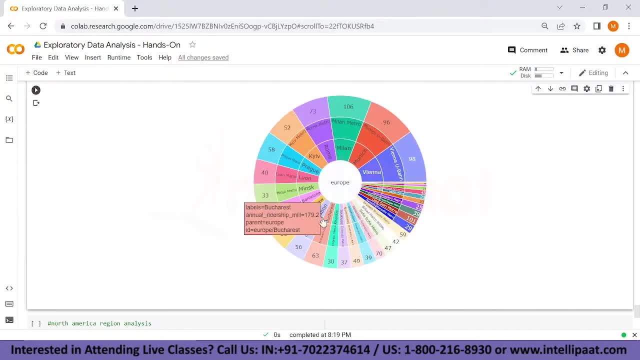 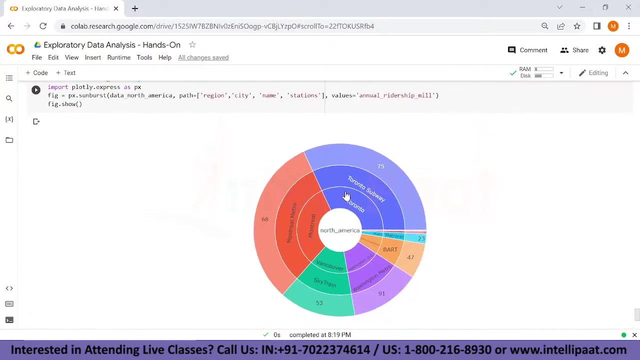 million riders every year. if we so far lil nealcom, vanzure, vin leva And Barcelona- we have for Vienna, Vienna actually has Vienna U-Bahn 98 stations with 459.8 million annual ridership. So if we take a look at this, Warsaw Metro we have, and similarly we've done that for North America also. 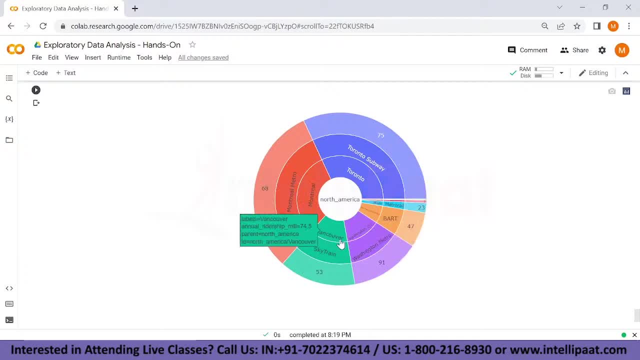 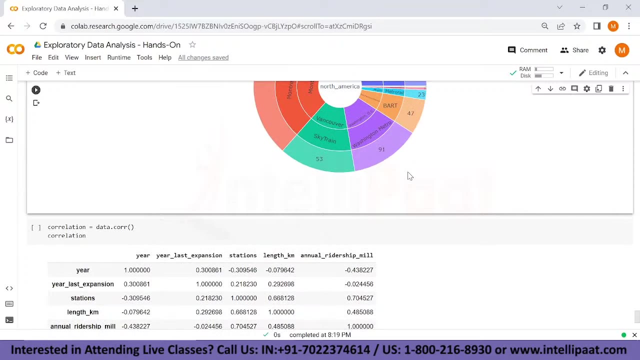 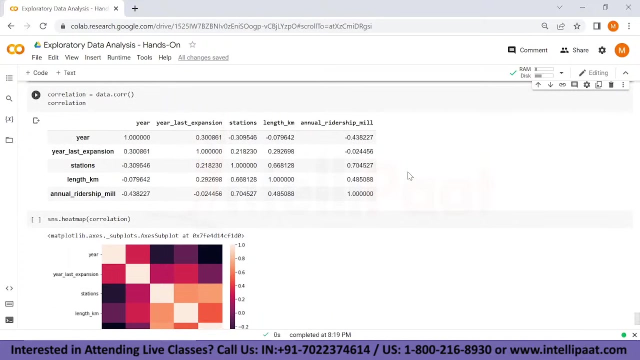 So we have Montreal, Toronto, Vancouver, Washington DC and there's Miami also, So a sunburst is something that you can use to get a clear picture of all the data points in your data set. Now, last but not least, I want to talk about the data correlation, which gives you a better picture of all the variables that are going to be correlated to each other. 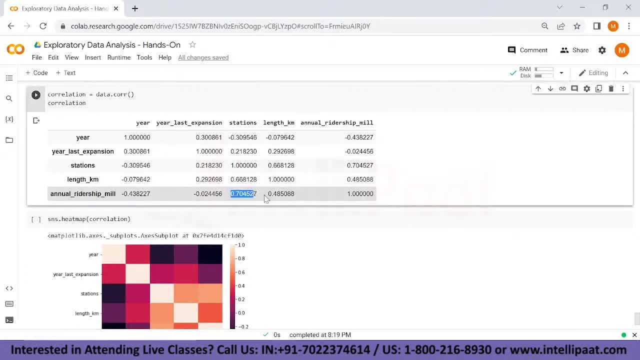 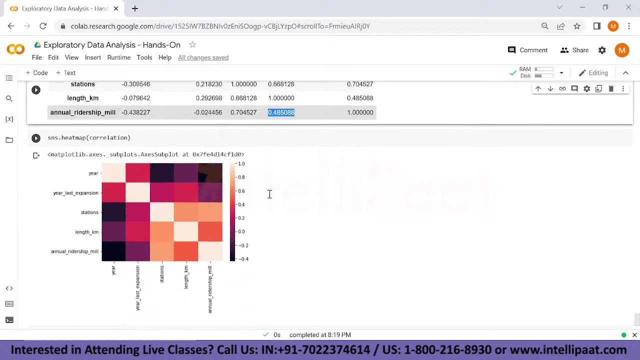 And if we check for annual ridership in million, we can see stations and length in kilometers is showing a positive correlation, where stations is actually showing a strong positive correlation, whereas length in kilometers is not that strong but is considerably showing somewhat correlated values over here for annual ridership. 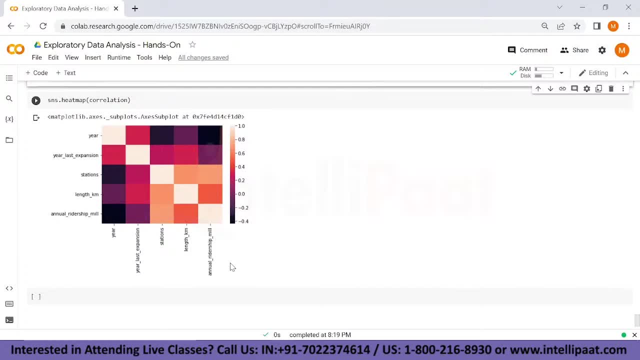 So this is where we are going to sum up our session. guys, If you have any questions, you can mention them in the comment section below. And, now that we have come to the end of the session, don't forget to subscribe to Intellipaat for more exciting videos. 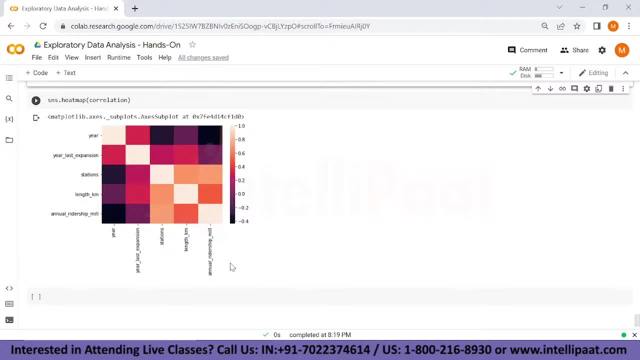 and press the bell icon to get the latest updates from Intellipaat. Also, tell us in the comments about your journey as an aspiring data scientist, which areas excite you the most and where we can help you master data science concepts in the best possible ways.